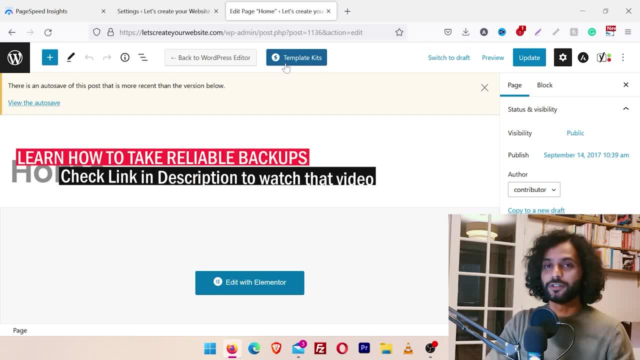 So, first thing, always take back your website, like always. if something happens, you can always restore your website. And if this plugin or any other plugin you are using broke your website, just deactivate the plugin. If you don't see changes, refresh the cache, because in most of the cases if you deactivate a plugin, all the effect of plugin will be gone. 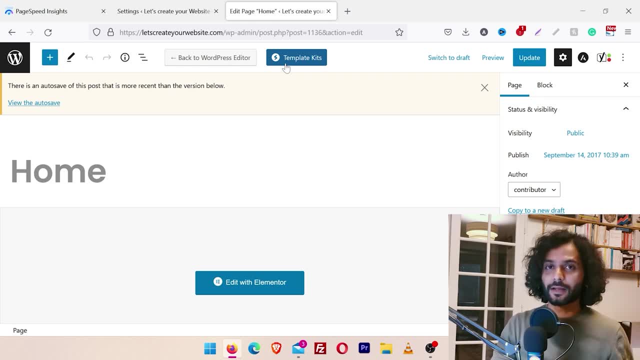 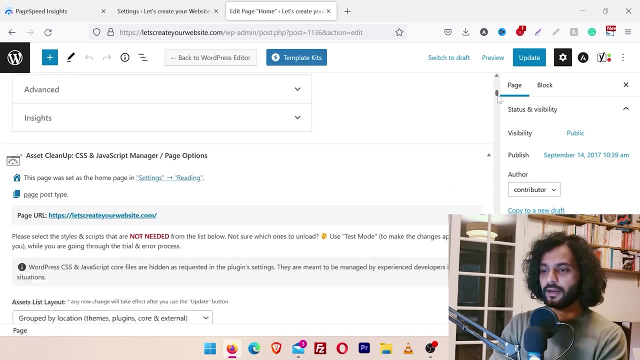 Your website will be back how it was before, And the best thing to always keep the backup before doing anything big on your website. With that said, let's see how this plugin works. Okay, so remember, we installed the plugin And now what you need to do is scroll your page. 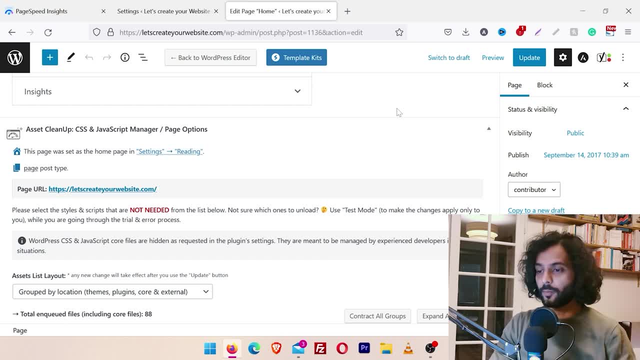 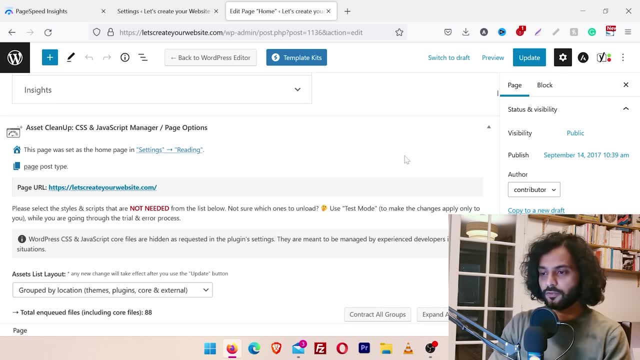 Just to mention again, we are doing this on home page of the website. Home page is the most important page. All other pages are important, but home page is the most important page. So once you scroll the page, you will find this option: Asset Cleanup section here. 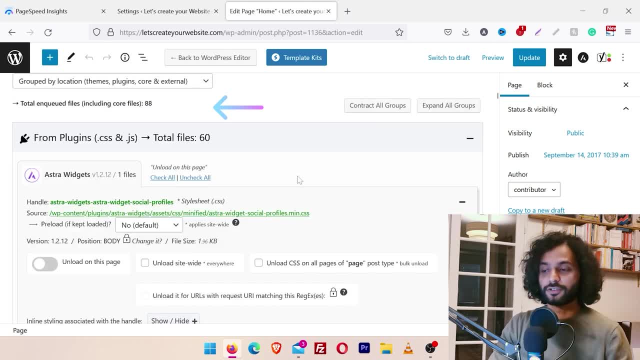 And here you can see all the JavaScript and CSS files which are loading on the page will be displayed here. It's going to take a little bit of logic and your knowledge about your website. So what we are going to do, we are going to remove unused CSS which are not used on that page. 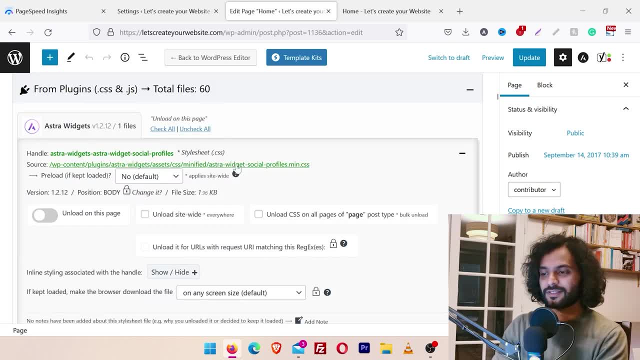 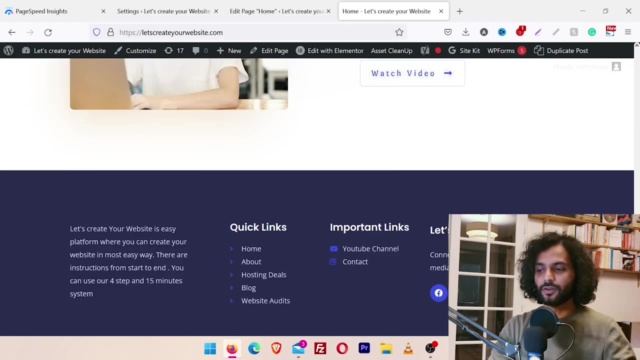 You will understand in a minute what I mean. You can see this CSS file which says extra widget: social profiles. You can make a logic that this CSS is used to display social profiles. If I go back to my website and I scroll the page, you can see I do not have any social profile element on my home page. 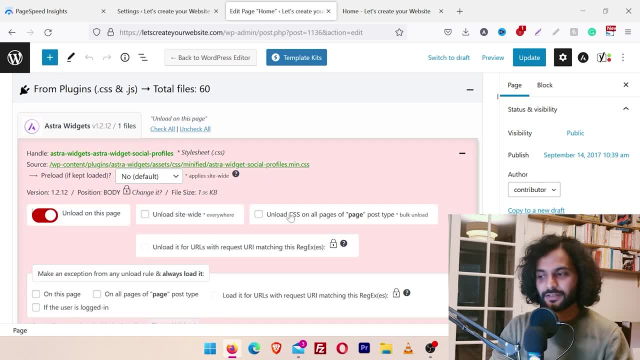 So what I will do? I will go back here. I will click on Unload. I will click on Unload on this page. So by doing this, we are unloading CSS file which is not used on that page. Normally, you are not using social profiles on every page. 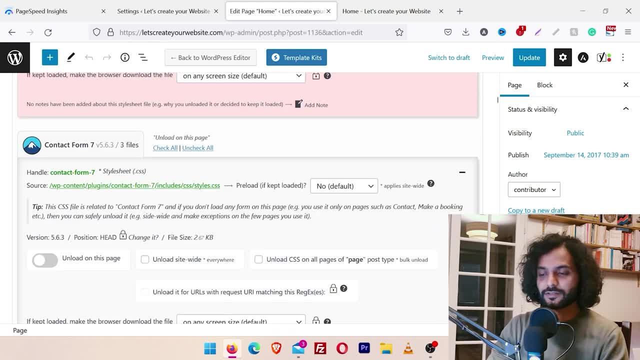 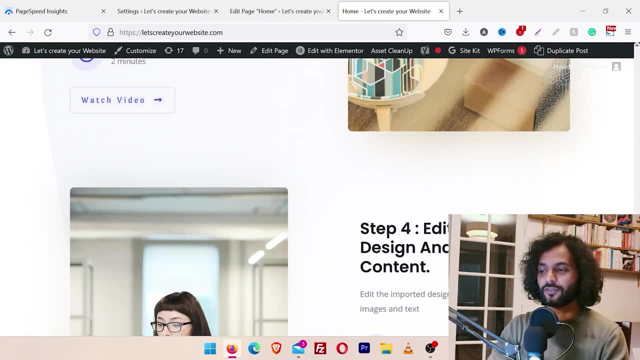 Let's take another example. If I scroll the page more, you can see this CSS file is added by contact form 7, to style the contact form. If I go back to my website, I do not have any contact form on my home page. 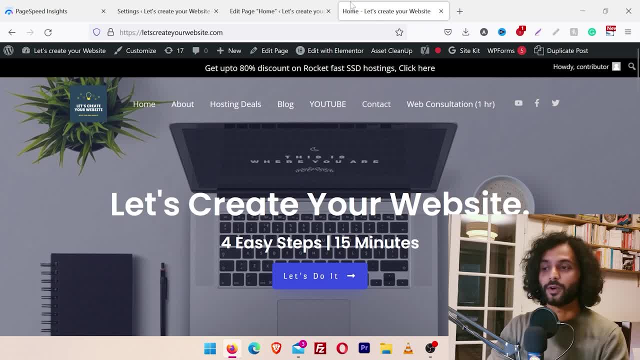 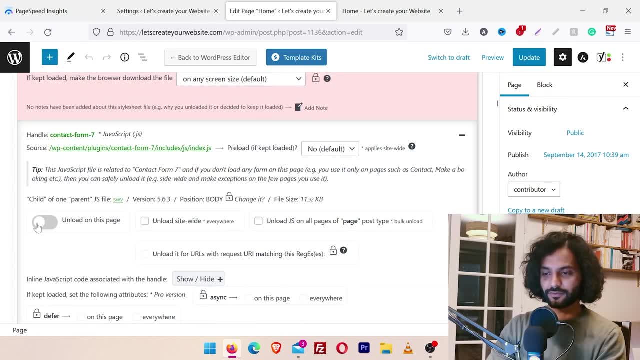 I have contact form on my contact page but not on the home page. So what I can do, I will just go here and I will unload on this page. If I scroll more, you can see there is another JS file added by contact form 7, which I am not using on home page. 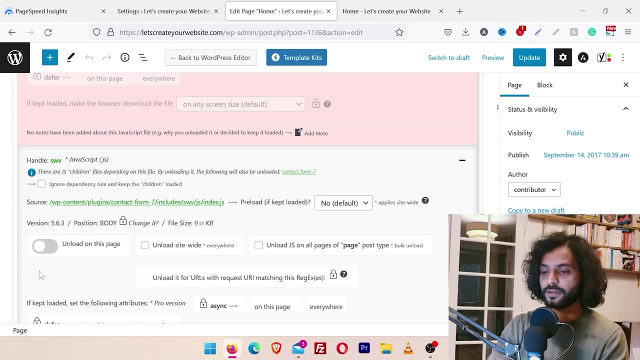 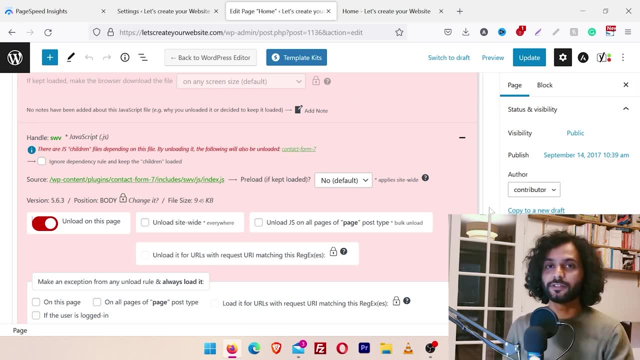 So I will unload this also. Basically I am not using contact form 7 on my home page, So I will unload all the contact form 7 files from my home page And when you make changes here on particular pages, they will be just affected on that page. 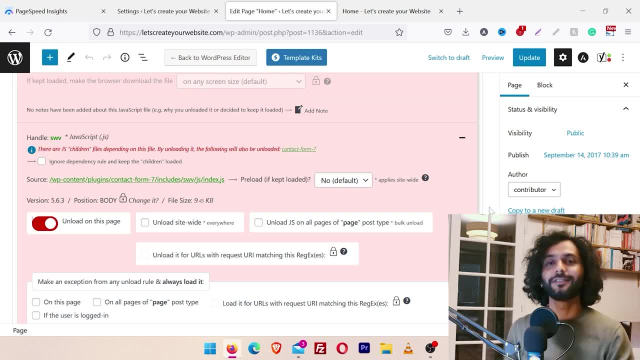 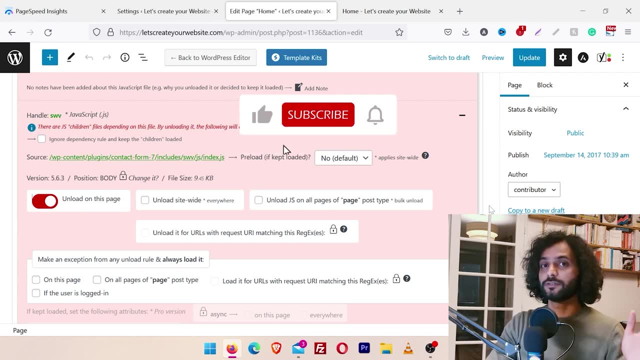 It will not be affected on other pages. So if I unload the scripts here, they will still load on other pages, but not on the home page And, as I said, I will create another video, which will be more in-depth video. how to remove CSS file manually. 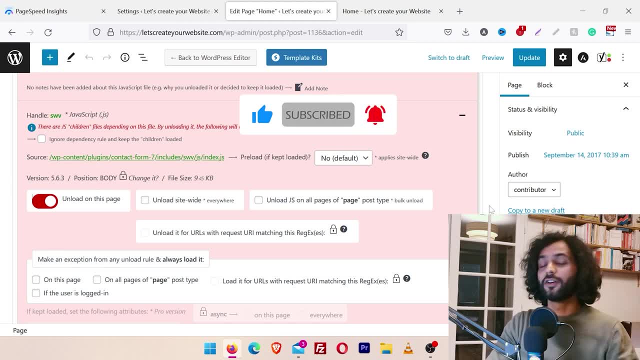 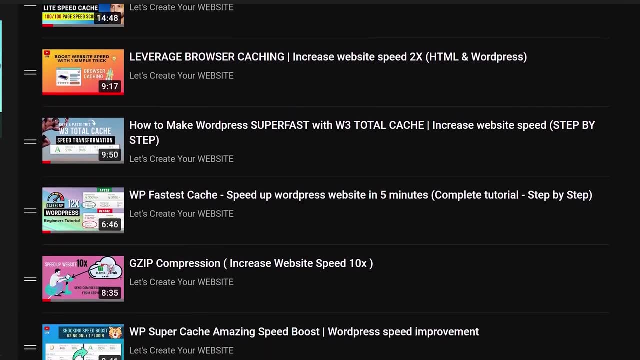 which will be more effective. But this is an easy method. It will work on most of the website. And now you will ask me- I create a lot of speedy prepare videos- why you need to use this SSCleaner plugin. Because sometimes what happens? every website is different and every website got different scripts. 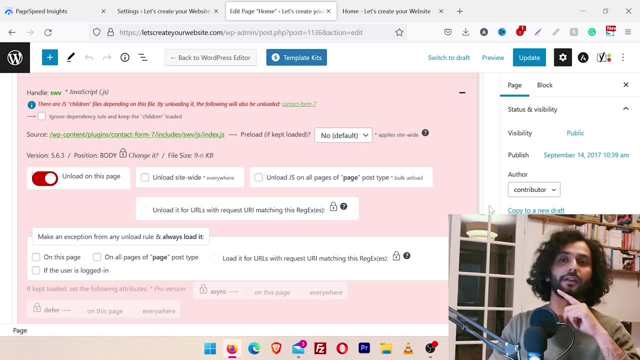 Sometimes you need to try different kind of methods. So if you have watched my Lightspeed video, I will put a link here, or any other video. you will find the link on the top somewhere. If they are not working for you 100%, you can use this plugin on the top of those plugins to get the best scores for Google PageSpeed. 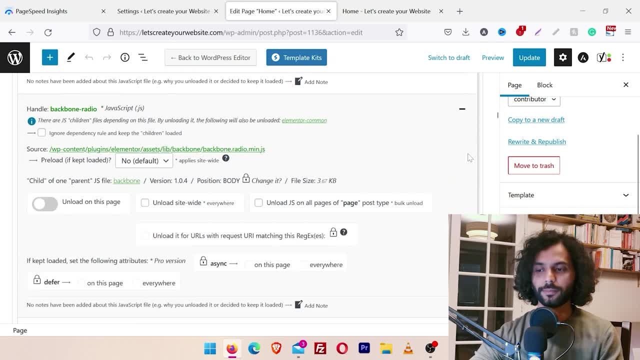 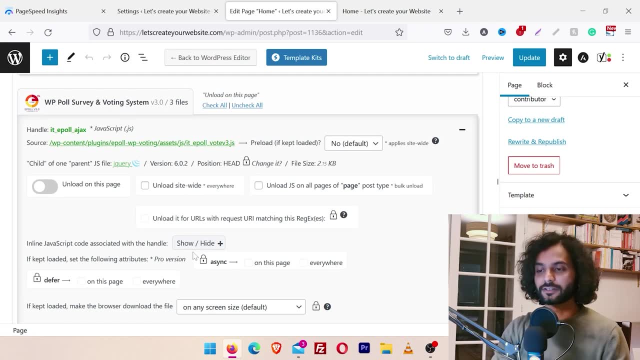 Okay, Let's scroll the page again And like this: you just need to scroll the page and find which CSS or JS you are not using on those pages And just unload them there. If you see, here I have another script, which is WP Poll Survey and Voting System. 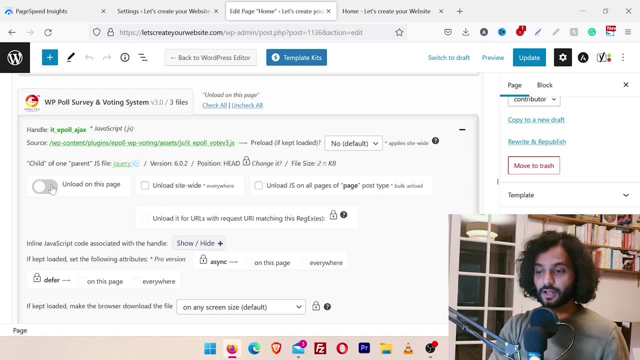 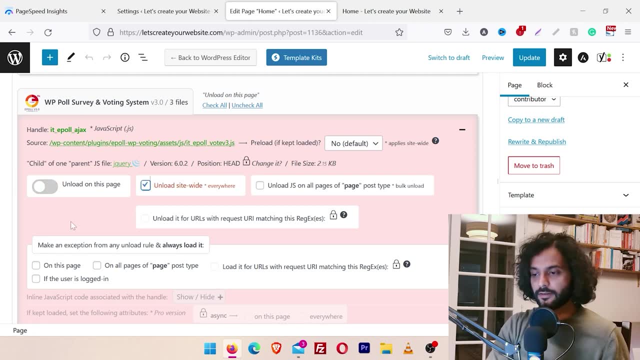 I am using this script just only one page on website, So I can 100% unload this script on the page. Even you can use some options like unload site-wide, So this script will be unloaded site-wide completely on your website. And what you can do when you unload site-wide: you can go the page where you are using this script. 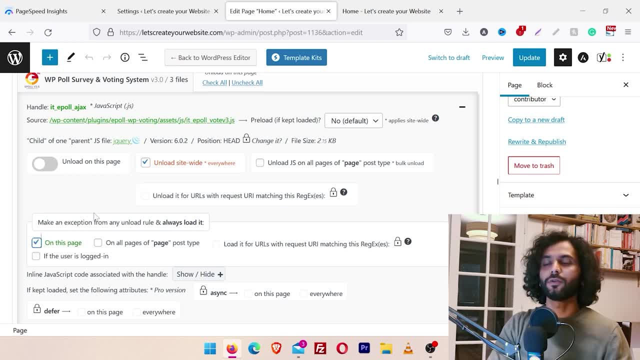 And then check this option. On this page, you can make an exception to load the script on particular pages. So like this way, you can really save lot of CSS and JS loading on your website, which will make your website really fast. 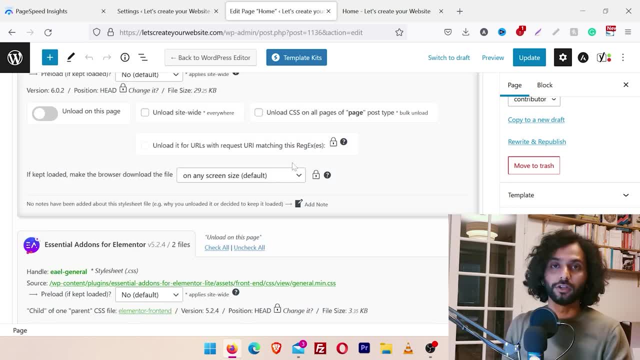 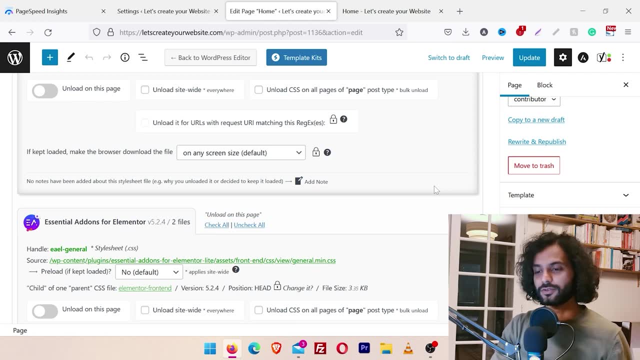 You can repeat this process for all the scripts which you are not using on all the pages. I am sure you will find lot of scripts which you are not using on all your website, And once you find all the CSS and JS you are not using on those pages, just click update. 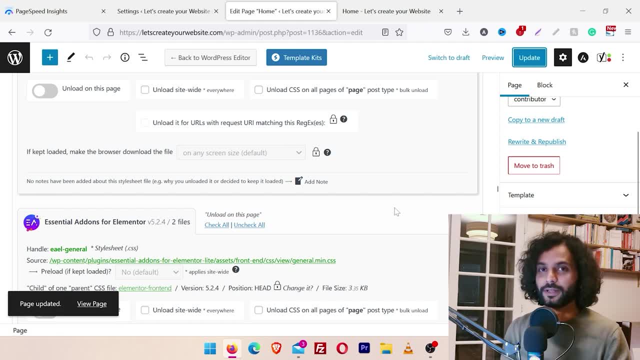 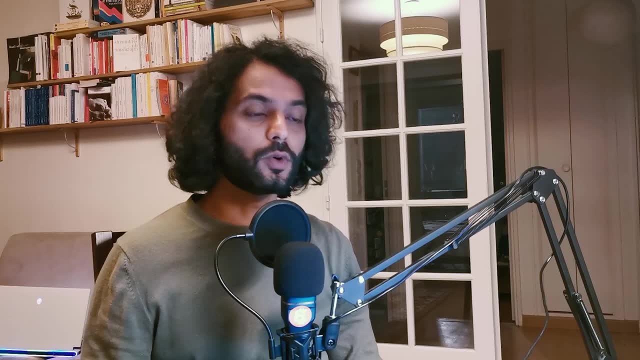 Now all these files we just unloaded. they will not load on your homepage And this will make your website score really high. This will take some time, But I am sure this will really help you to improve your website page speed scores. And if you want to know how I got 100 out of 100 for Google page speed scores, check out this video on screen. 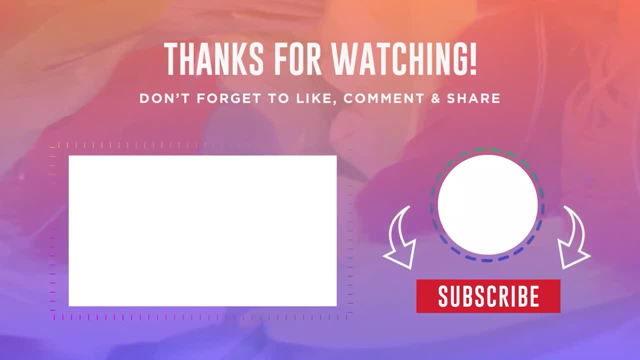 And don't forget to give this video a thumbs up and subscribe to this channel And share this video with somebody who might need it.